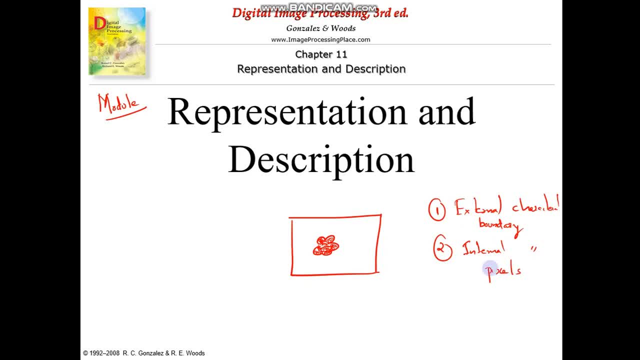 when primary focus is on regional properties such as color and text. In that case, we take the pixels. 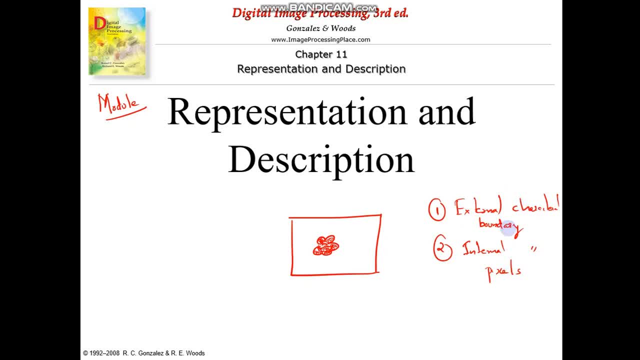 Okay, whereas in external characteristics, the more focus is on the shape. 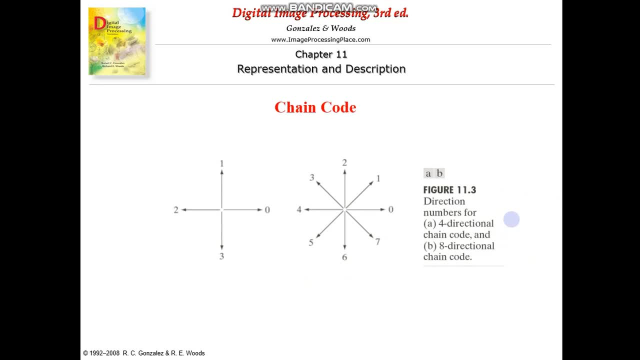 So, we are talking about the shape. So, we are talking about the shape. So, we are talking about the shape. Now, moving on to the first method that is chain code. 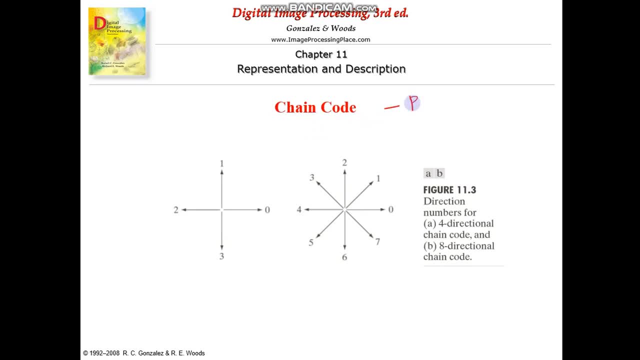 So, chain code is used to represent a boundary. It is used to represent a boundary. So, external. 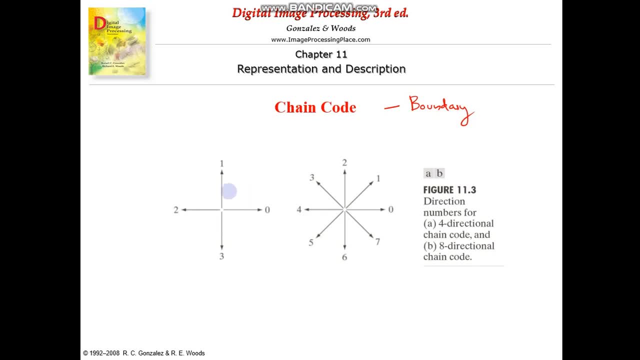 Using a connected sequence of straight line segments. 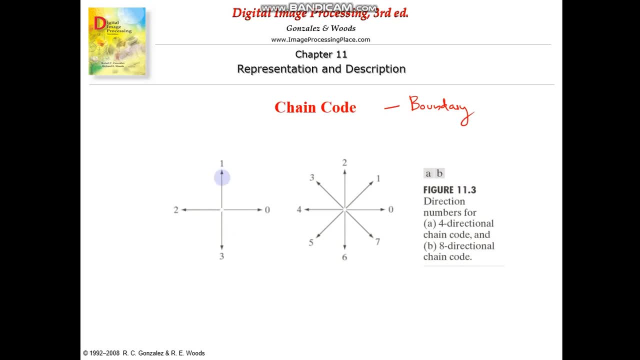 So, these are some straight line segments and each direction has got a number. So, 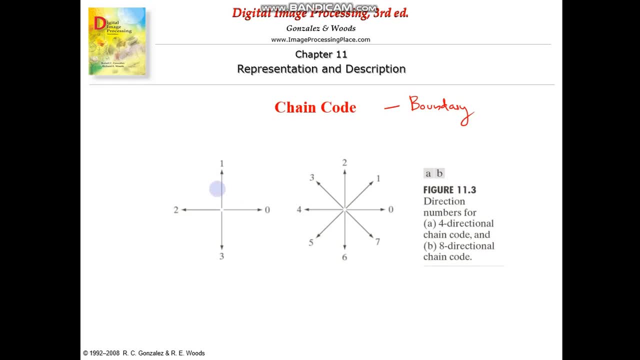 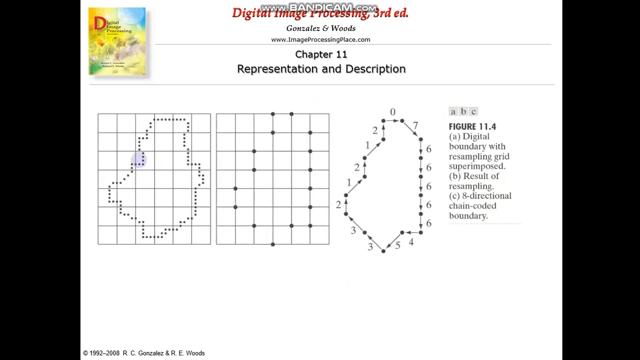 This representation, okay, this representation based on line segments depends on four directional or eight directional. That is, we already know about the four connectivity and eight connectivity. Okay. So, this choosing this depends on four connectivity or eight connectivity of the segments. Okay. And we have a numbering, numbering scheme for each direction. Okay. So, we, what we do is we acquire digital image and they are processed in a grid format. See this, we have some boundary and they are processed in a grid format. This grid format may not be equal to the pixel. Okay. And we approximate the shape. We approximate the shape to the shape of the grid. Okay. This is the grid format. 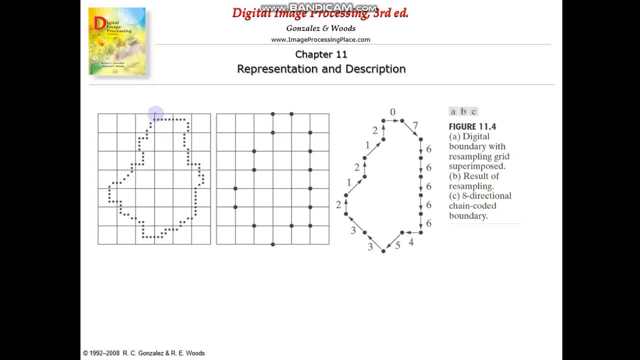 This is the result of approximation. Maybe this shape we will approximate to this point. Okay. See, depending upon the algorithm we are using, we can take. Okay. So, in the resultant here, they are not taking this. So, we can take it here. So, we are approximating to the shape as given in the output here. Different algorithms may give a different approximation. Okay. 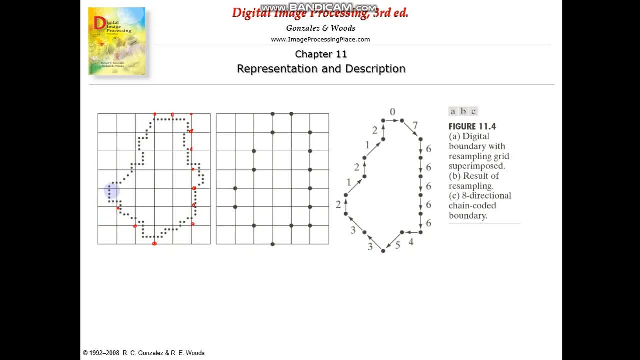 We will choose this one. So, here, here is the, the same approximation. So, we are approximating to the nearest, nearest point. Okay. So, here, this point, these two points. Okay. These points, they are avoiding. So, let me drop it. 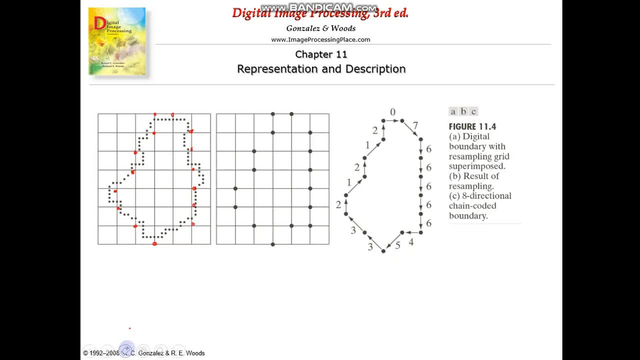 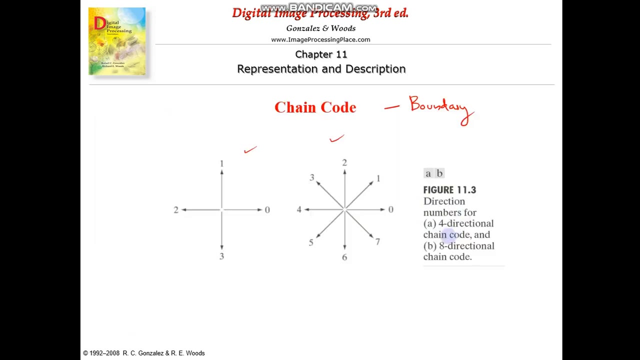 Now, so, in the grid-like pattern, we approximate the shape. Okay. Now, depending upon whether we are following four-directional chain code or eight-directional chain code, we are giving a number for each grid. Okay. Now, what to do next? So, the chain. 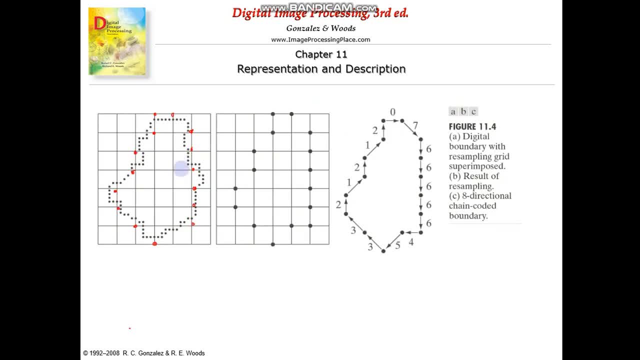 So, the chain code, we can be generated by following a boundary in a clockwise direction. So, follow a clockwise direction. So, by following a clockwise direction. Okay. Put an arrow here. Now, okay, here is the way. Okay. Now, see this. Here, we can connect like this. 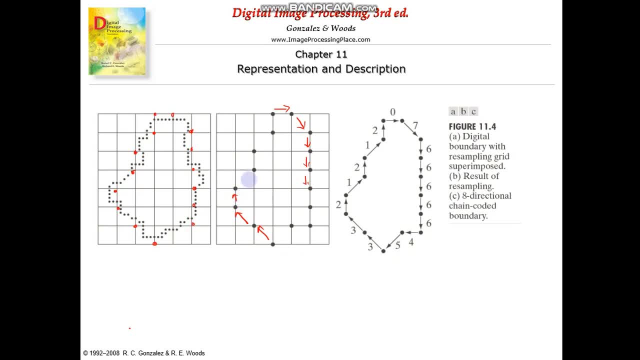 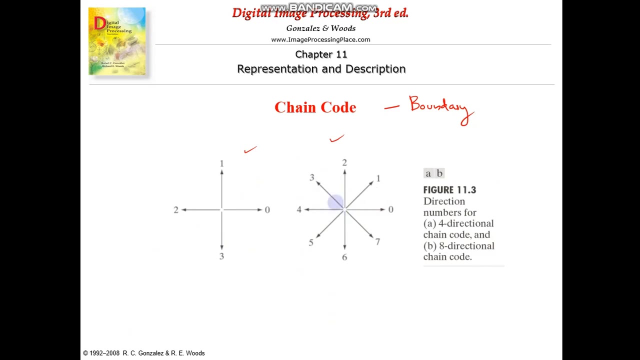 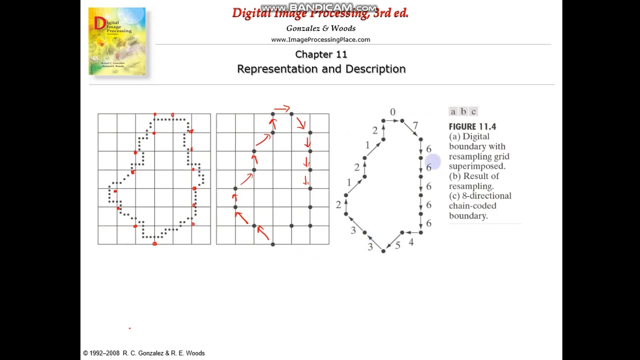 Now, throughout this image, you connect to get the shape. Now, if it is 8 directional chain chord, okay, we can follow this numbering, okay. This is 0, 1, 2, 3, 4, 5, 6, 7, okay. 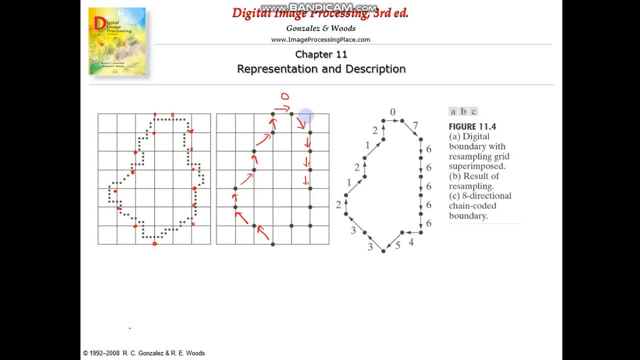 So, this is 0, here it is 7, depending upon that number, okay. 0, 1, 2, 3, 4, 5, 6, 7, okay. Give an arrow also, when it is easy. 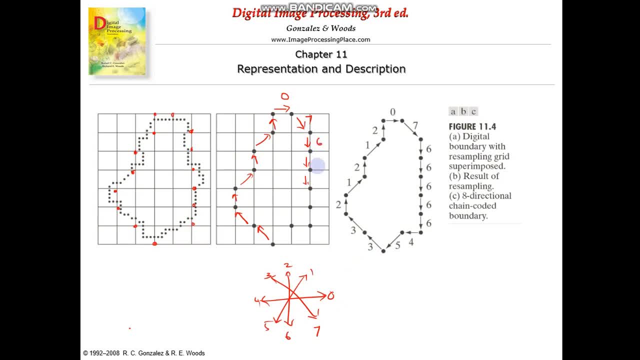 So, now 6, 6, 6, 7, okay. 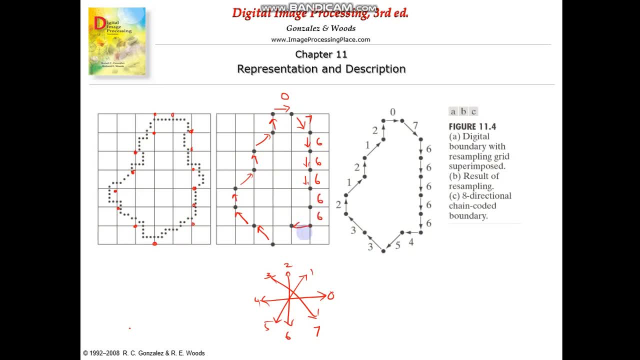 6, 6, now here, okay, 4, then this shape, 5, then 3, 3, then up, 2, then 1, then up, 2, 1, then up, it is 2.